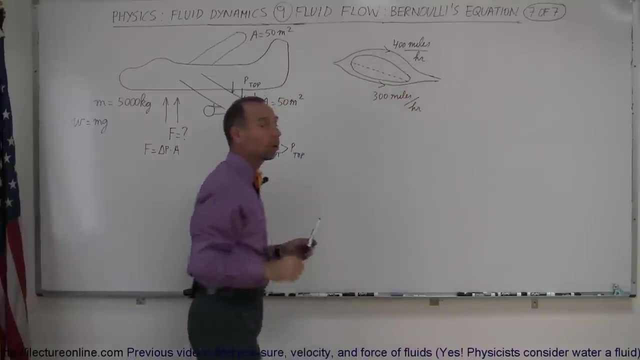 of the wing. Air will flow above the wing and air will flow below the wing, And it turns out the wing is shaped in such a way that it's more bulging at the top than compared to the bottom, And so the air that has to flow over the wing has to travel a greater distance than the air. 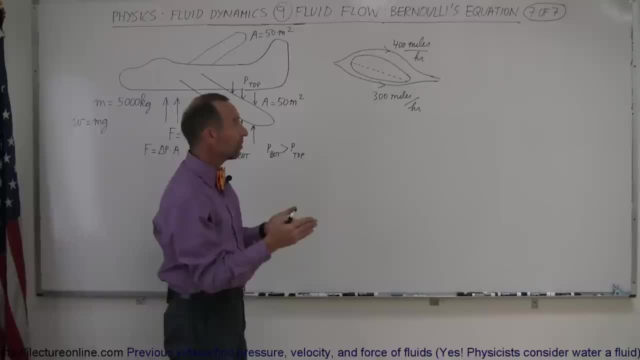 that has to travel below the wing, Since it has to travel a greater distance in the same amount of time, because eventually all the air molecules have to make it the other side of the wing. they just don't disappear, they have to stay there. the speed of the molecules above the. 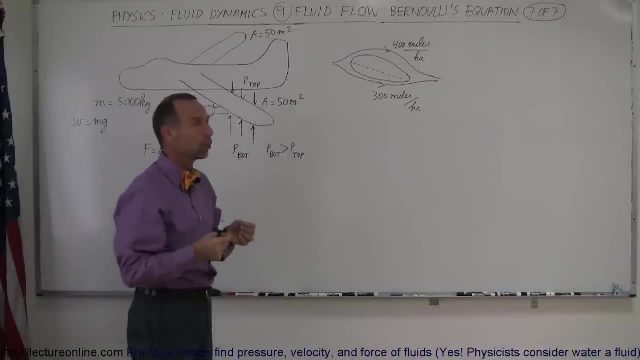 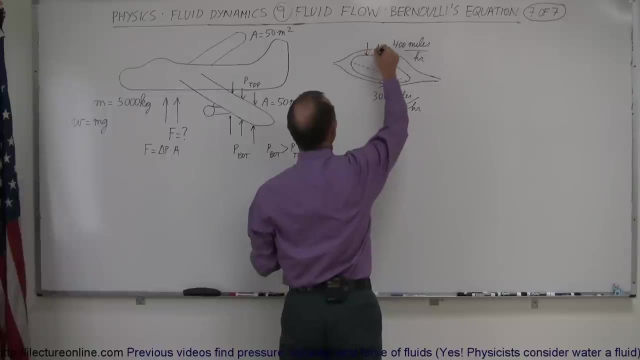 wing is greater than the speed of the air molecules below the wing, And since the speed is greater above the wing, there's less pressure above the wing. so less air pressure pushing down, More air pressure pushing up, and it's the difference in that pressure that causes the 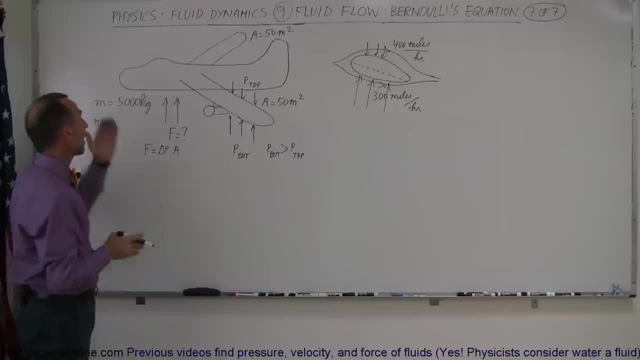 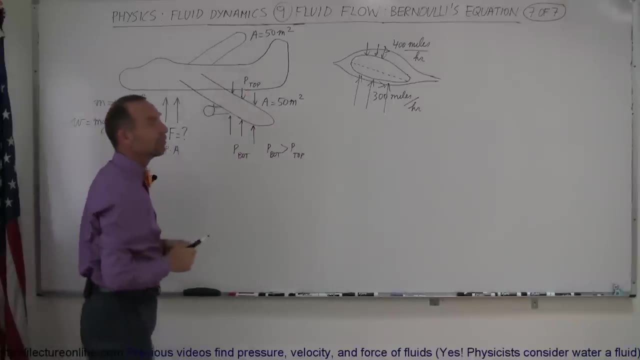 airplane to stay in the sky. So let's say, for an example, we have an airplane, it has a mass of 5,000 kilograms and it has wings, each of them with an area of 50 square meters. And let's assume 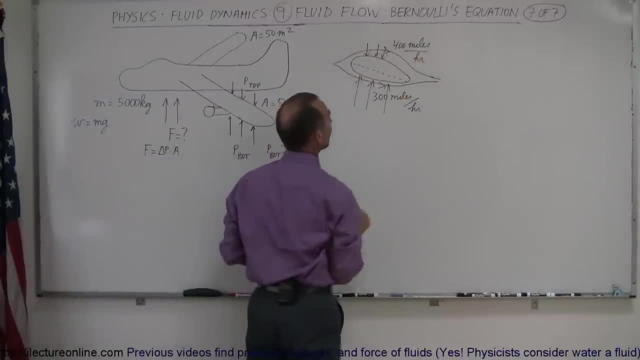 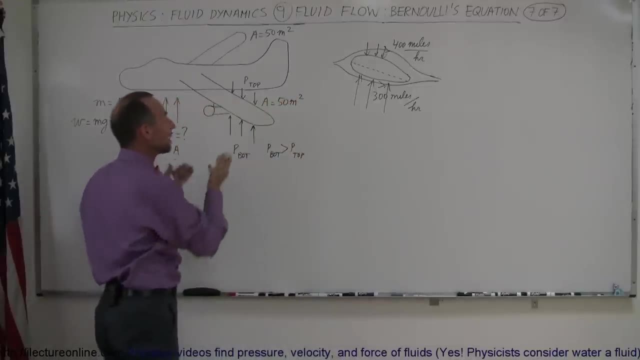 in our example, that the air above the wing moves at 400 miles per hour and the air below the wing moves at 300 miles per hour. Will that cause enough of a pressure difference to keep the airplane in the air? Now, I haven't worked out this problem yet, so I don't know. I'm kind of curious, so let's. 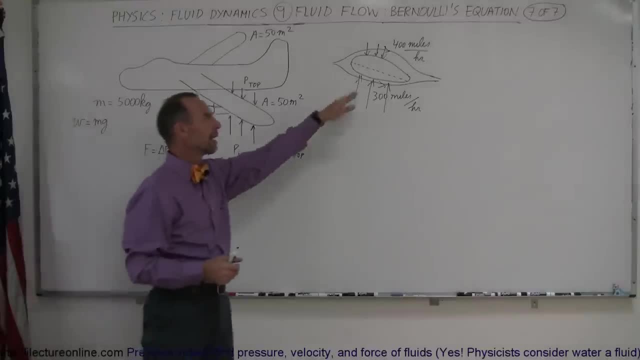 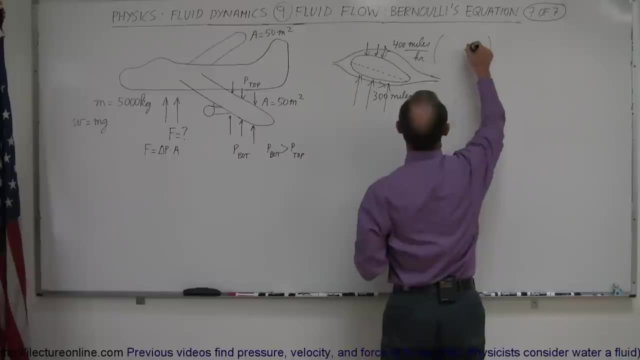 go find out. Well, first, before we get started, let's convert the miles per hour into meters per second, and to do that we have to go like this. This is equal to: let's say, we need meters at the top, we need miles at the bottom, and one mile is 609 meters. and then 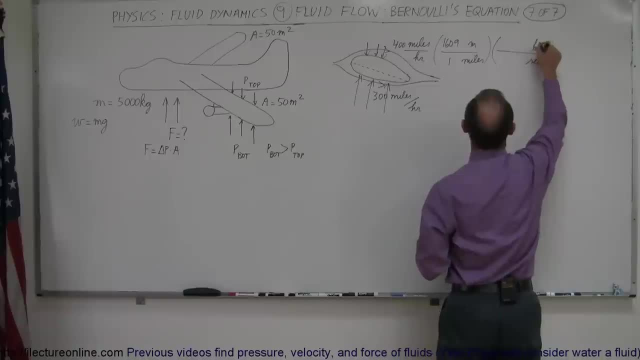 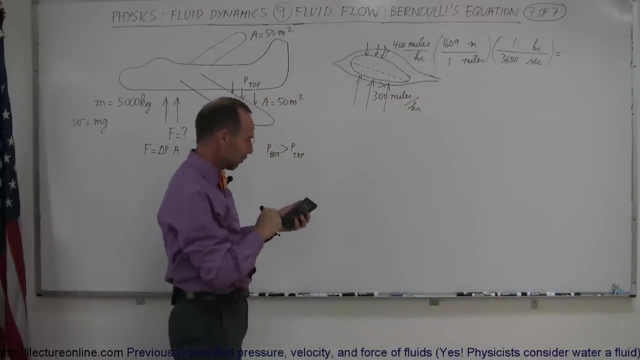 we have to convert to seconds. we need seconds at the bottom hours, at the top, one hour is 3,600 seconds. So let's see how many meters per second we have to convert into meters. Meters per second, that is. so we have 400 times 1609, divided by 3,600, and it looks 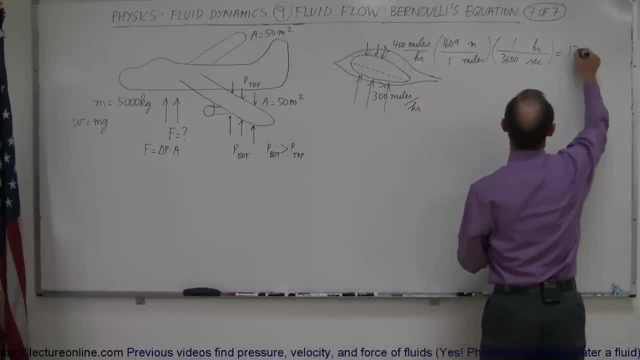 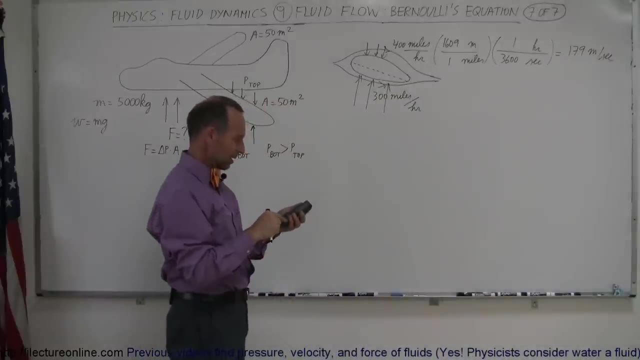 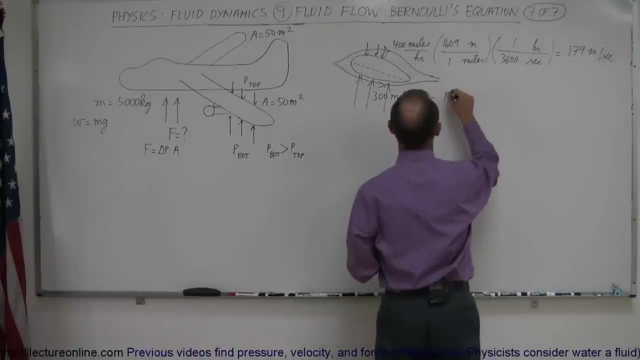 like 170, let's just call it 179 meters per second, And then for 300 miles per hour. so that's divided by 4 times 3 equals and that would be 134 meters per second. so this would be 134 meters per second, Oop, not per second. 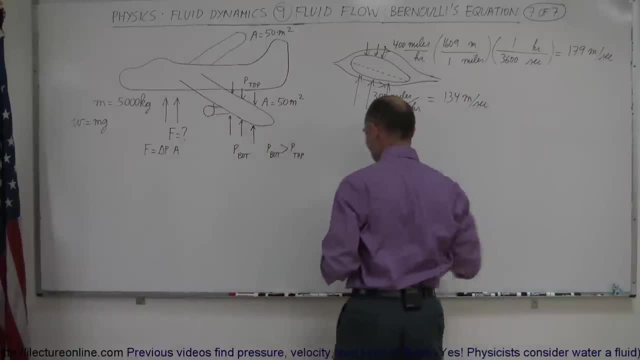 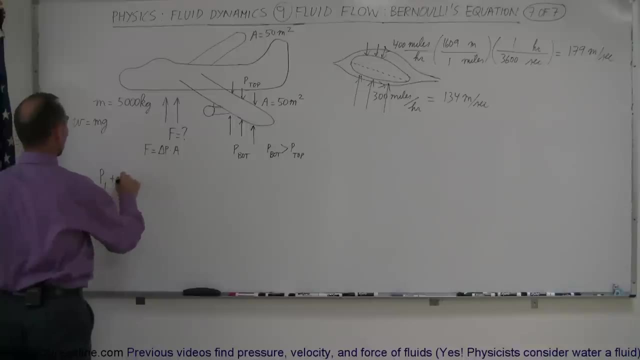 Not per second square, but simply per meters. Okay, so now we're going to use Bernoulli's equation. So to do that we write: P1,, pressure 1, plus rho, GH1 plus one-half rho, V1 squared. 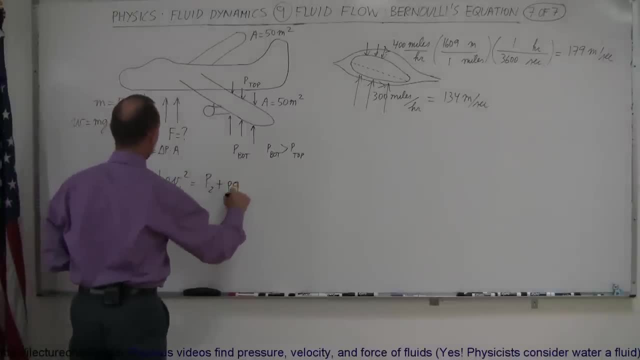 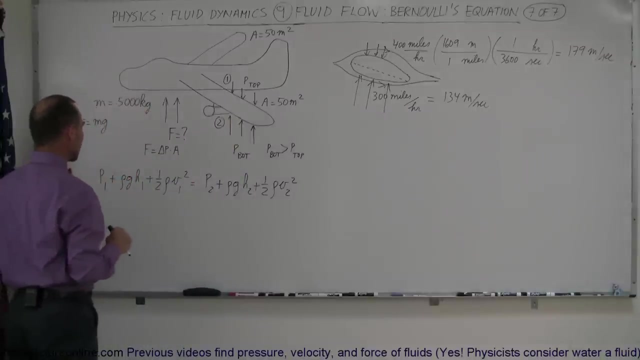 is equal to pressure 2 plus rho GH2 plus one-half rho V2 squared. and now I have to pick a 1 and a 2, let's call 1 above the wing, let's call 2 below the wing, All right. So let's see here, Since the height above the wing compared to below the 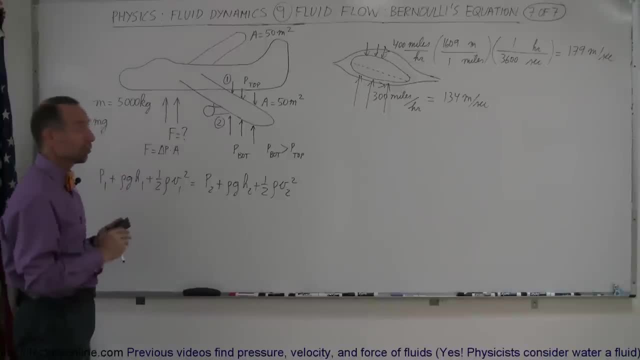 wing is just a few feet, just a meter or so, it doesn't really make any difference, because the air, you know, the air pressure relative to the height, will be very, very similar above and below the wing. We could probably just go ahead and ignore these two terms, So just. 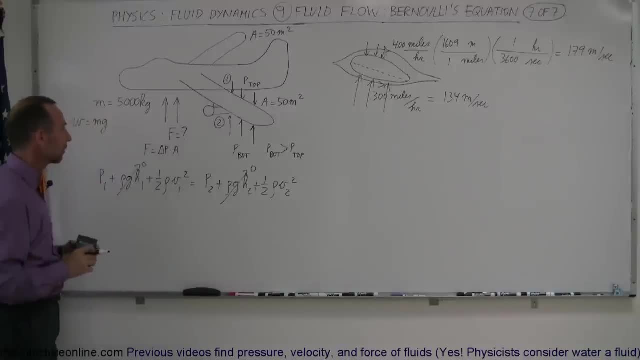 get rid of them. If you subtract them from each other, you can just simply get rid of them. Now We want pressure 1 minus pressure 2.. Now we expect pressure 2 to be greater. so I'm going to solve this whole equation for pressure 2 minus pressure 1.. So I'm going to move. 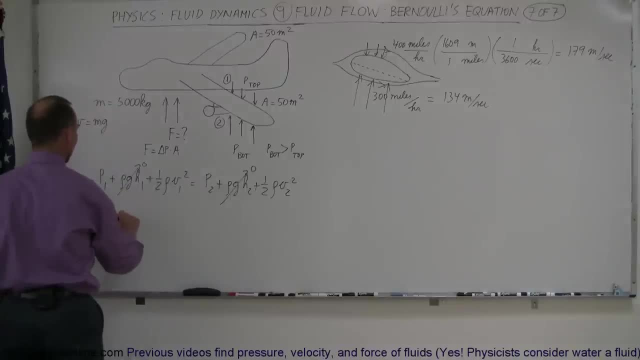 pressure 1 over here and move that over here. So we have one-half rho V1 squared minus one-half rho V2 squared is equal to pressure 2 minus pressure 1.. Remember we expect a greater pressure at the bottom than at the top. 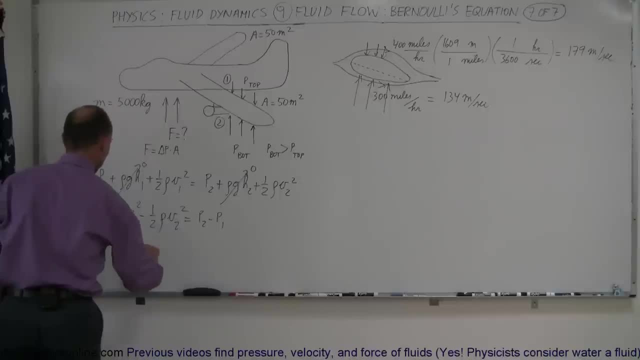 Flipping the equation around, I get pressure 2 minus pressure 1 is equal to, and factoring out a one-half Times rho, I'm left with a V1 squared minus V2 squared. So this will give me the pressure. 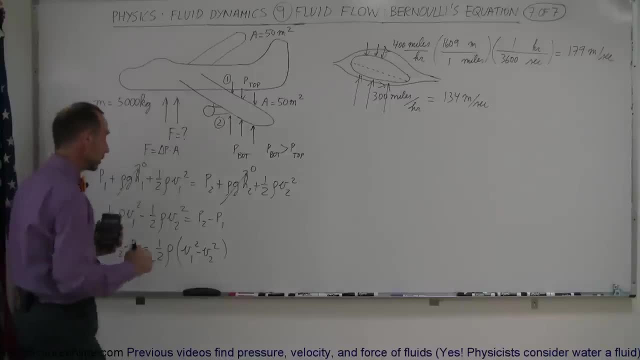 difference above and below the wing. All right, Plug in the numbers, This is equal to one-half times the density. Now let's take the density at sea level, and then of course you can imagine, as the plane goes higher and higher and higher and the density gets smaller, that 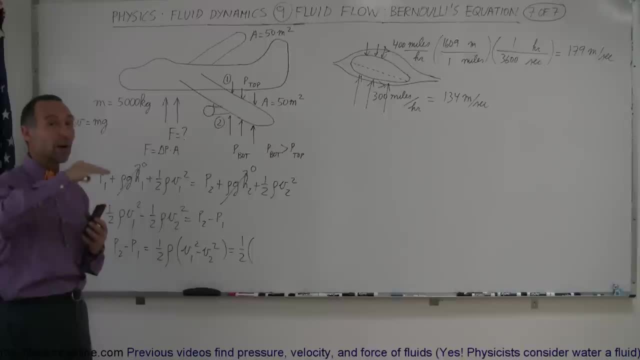 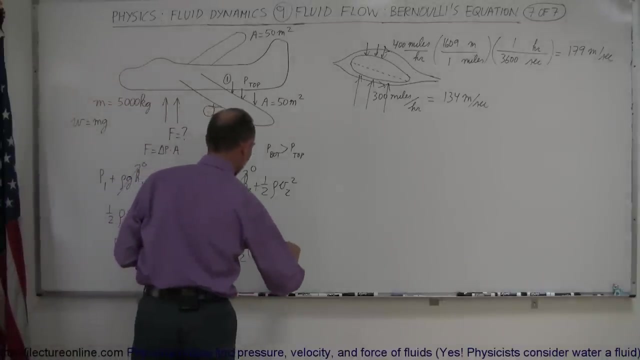 also means that the pressure difference will get smaller. So there's a limit as to how high planes can fly before the air gets so thin that the difference in pressure is no longer sufficient to keep the plane in the air. So let's just simply call the density here. at sea level That would be 1.29 kilograms. 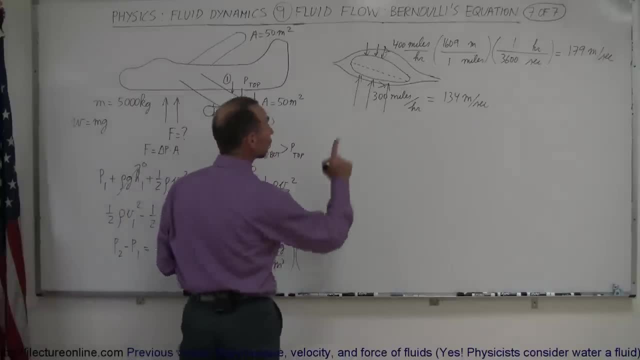 per cubic meter And then multiply that times V1. squared Now, V1 would be- let's see the V at the top- that would be the 179 meters per second Square that, And oops, I'm not. 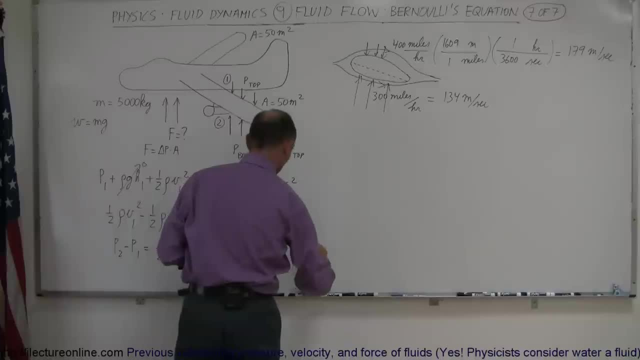 dividing anything here. Let me write that again. So it would be 179 meters per second. You have to square that like that, minus the speed at the bottom, which is 134 meters per second, and we have to square that as well. 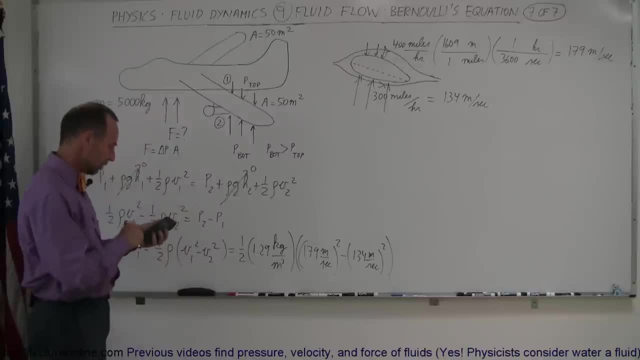 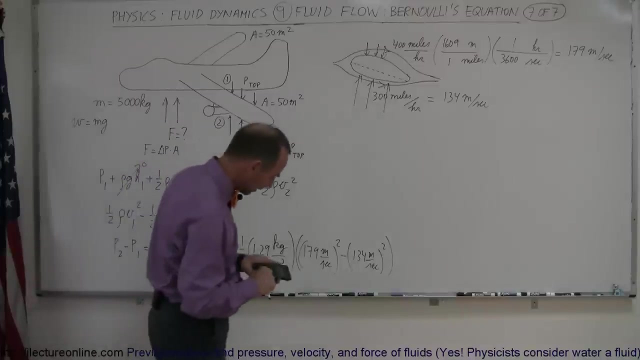 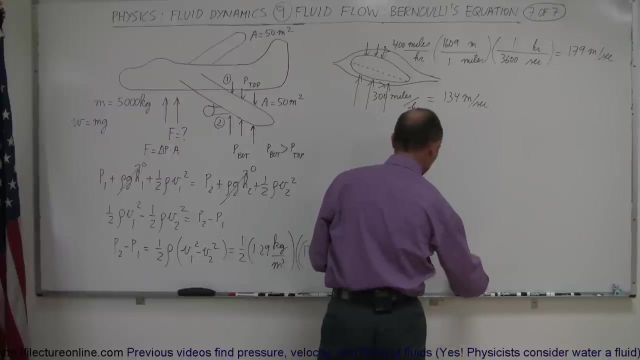 All right, so let's do that now. So 179 squared minus 134 squared equals multiple at a times 1.29 and divided by 2. And what do we get? So I can see that this is 9,085 newtons per square meter. 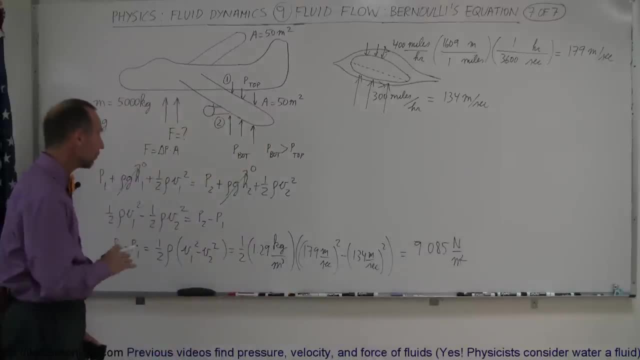 All right, so that would be the pressure difference between the top and the bottom. Now, what would be the total force? Now, the total force on the plane pushing the plane up, would be the pressure difference times the area of the wings. 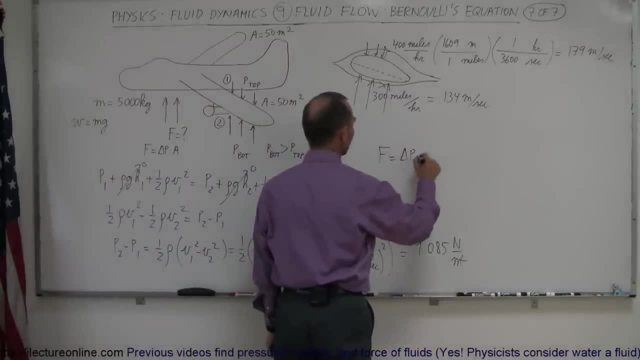 So the force is equal to the change in the pressure times the area of the wings. So the difference in the pressure times the area, The difference in the pressure, is 9,085 newtons per square meters Multiple at a times the area. 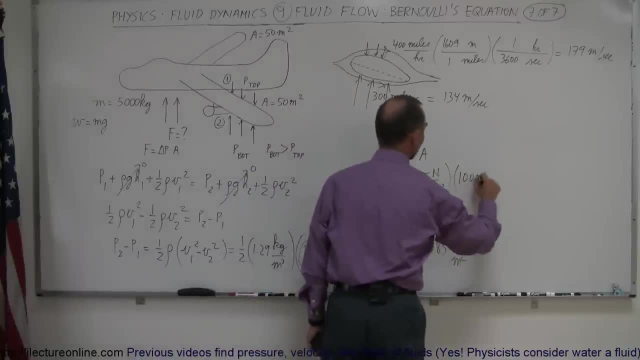 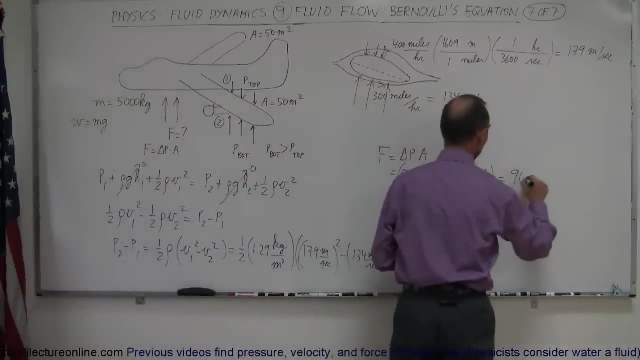 The area would be 50 plus 50, or 100 square meters, 100 meters squared. And so what do we get? Hmm, 100 times 9,000, that would be 908,500 newtons per square meter.